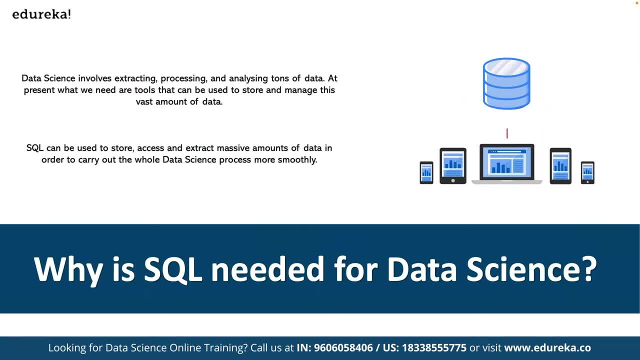 tons of data and at present what we need are tools that can be used to store, manage and process this vast amount of data that we have the access to. so sql can be used to store, access and even extract information. that means we can use it to perform all the credit operations that we have and that 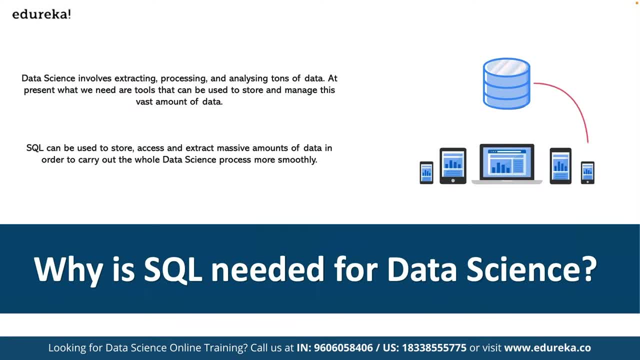 too, in massive amounts in order to carry out the whole data science process more smoothly. since many people developers, they are already familiar with this particular language, so they get familiar with how the entire process should be and how is that. it has pre-updated, so it becomes easier for them, for them to work on data science components. so if we talk about 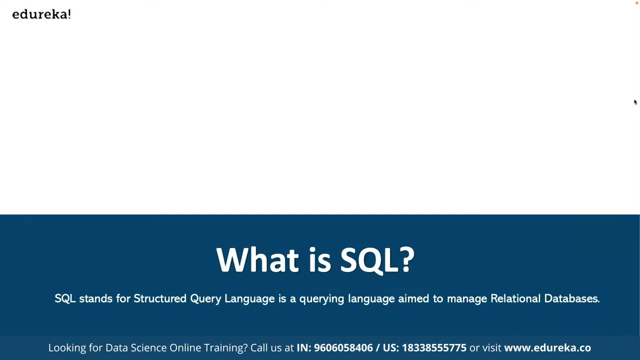 sql. so sql here is basically what? the structured query language, which is focused on manipulation of the relational databases, for example. if you talk about relational database, then we have data stored in the format of rows and tables where we can interpret that by using the different operations that we have. for example, if you are looking to update the entries in the 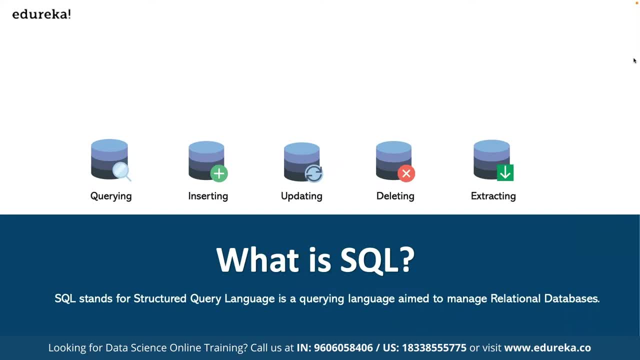 tables. then we can make use of sql. we are looking to perform some changes. or we can say: perform the editing, or we want to perform the deletion of the items. you want to update the items, so all the crud operations that we have. crud means create, read, update, delete. you want to extract this. 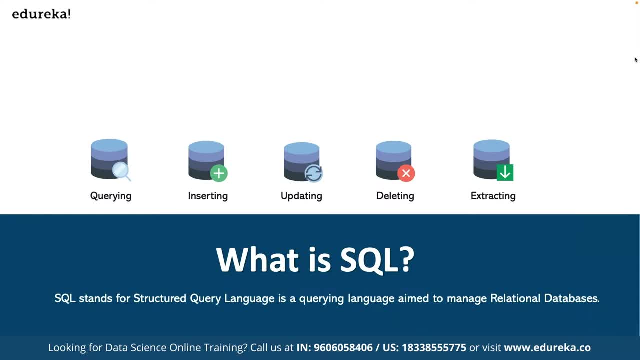 information. so everything is possible by using the database service here and that goes by the name of mysql, so there are multiple database engines available. so mysql is one of the database engine with one of the most popular database engine out there that we can use for data manipulation. 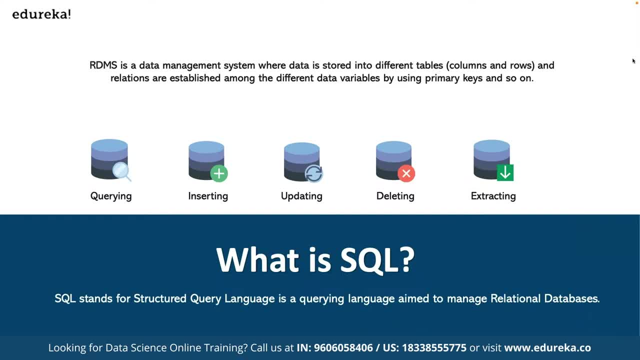 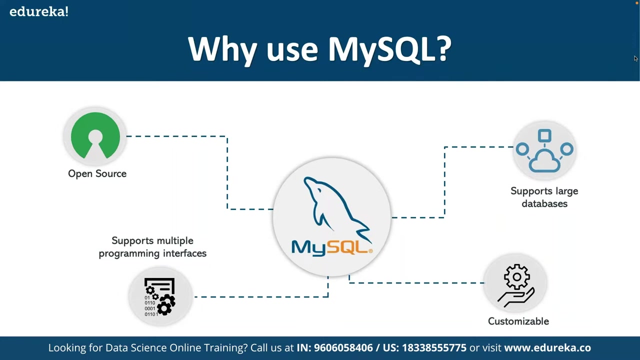 and rdbms is basically a data management system where data is stored into different tables, as we discussed, in terms of rows and columns, and the relations are established among different data variables by using the primary keys and the other components here step by step. so mysql has been one of the most popular database engine because of multiple reasons. first of all, 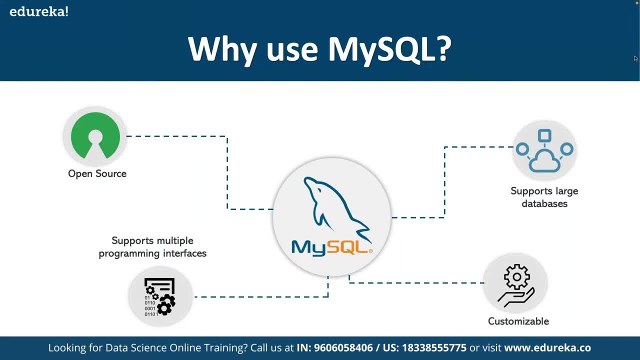 it is open source. that means there is no licensing involved here. then it supports the multiple programming interfaces. so we have we have the access to the cli. we can access it by using the gui method as well, and we do have the support to large databases, where we can create a good number of database or a single instance, as long as we 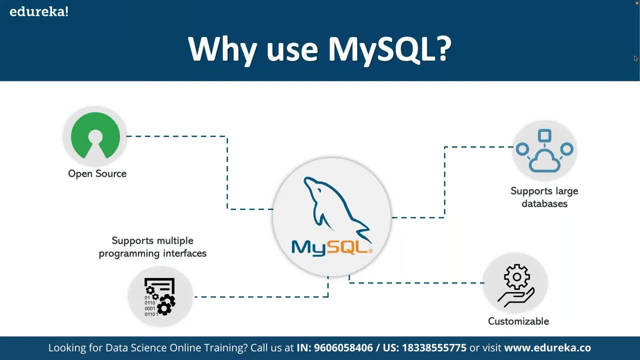 have the storage available, so we don't have a limitation of deploying this, just a single database or instance, like we have an oracle database engine, so we don't have a limitation like that. and then it is customizable so that we can customize it based on the requirement. now, in terms of the 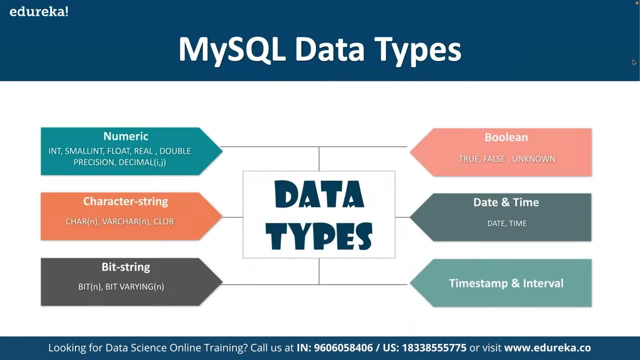 data types. there are multiple data types available in mysql. like we have numeric, we can go for character string, for bit string, for the boolean where we want to check for a given value, if it is true or not, then we have for date, time, timestamp and the interval. all right, then. so 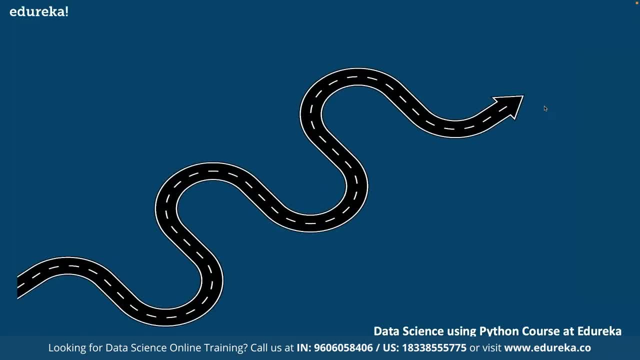 as a part of the structured training. either we, that we can get the data in the ender rica is, first of all, you are going to have a discussion on python, like having a complete hands-on on how python is structured, and then, in terms, here you're going to: 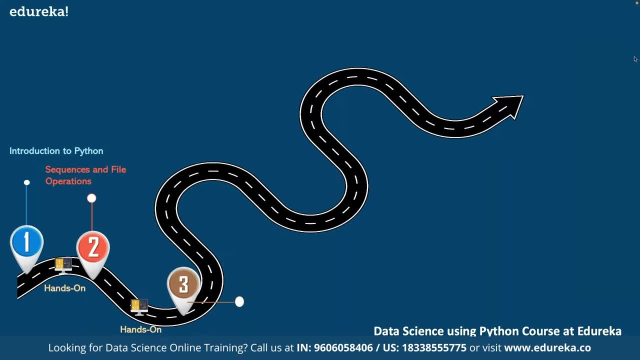 get this complete sequence and final component here, then we are going to learn on the functions, on oops modules, errors and exception. then you're going to get the discussion done on numpy, pandas and matplotlib. then you'll be having the access to data manipulation- how we can manipulate. 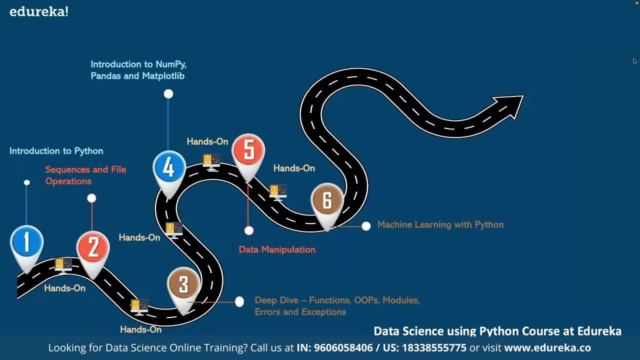 the data set and then we have the as a complete part that we can go ahead and follow towards the end. we can focus on model selection, boosting, to improvise the performance. so if you talk about the basics of sql, then again we can simply create the database. we can. 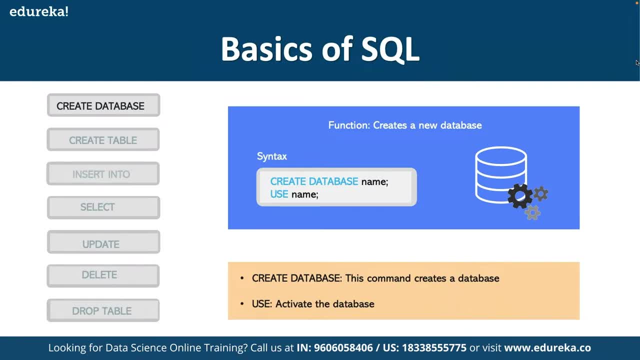 create a table, we can insert the entries into the table, we can perform the we can say update, by selecting the data in the given table and again deleting and dropping it as well. so let's do one thing first of all: let's get connected to a database that we have deployed in one of the 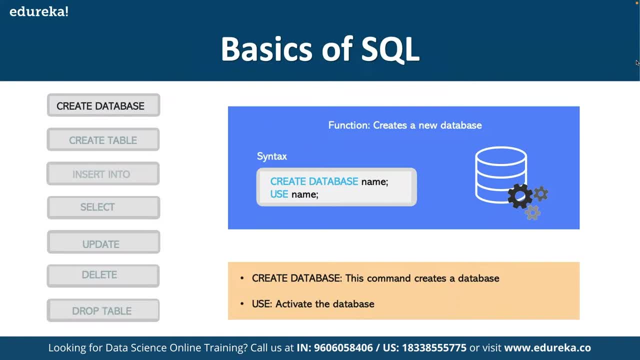 cloud platforms. so right now we have used our aws cloud to deploy a database instance running my sql database engine and by using one of the database line we are going to get connected to it. so here we are going to get connected to a remote database engine that we had deployed on aws and 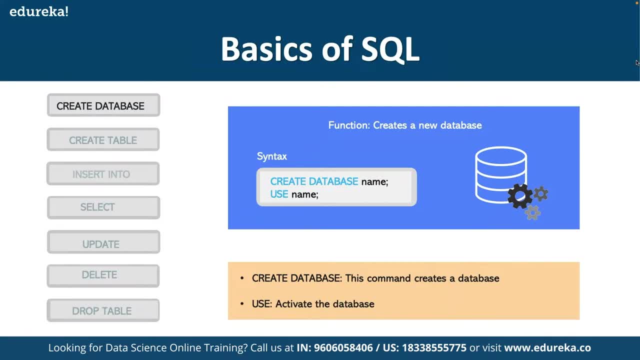 for that we are going to make use of different clients. for example, if you are comfortable working with, let's say if you have deployed, to suppose, mysql, so you can either use mysql workbench or you can go ahead and make use of hidea sql as well, you can use the mysql workbench as well. 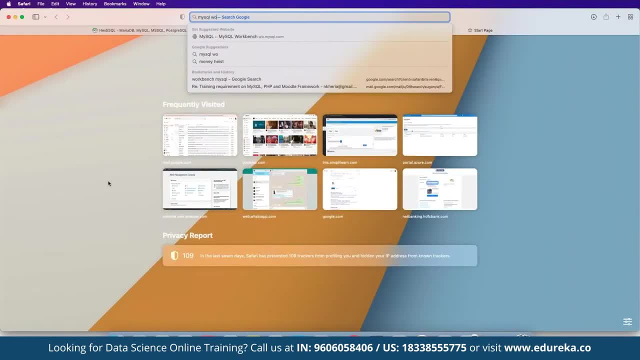 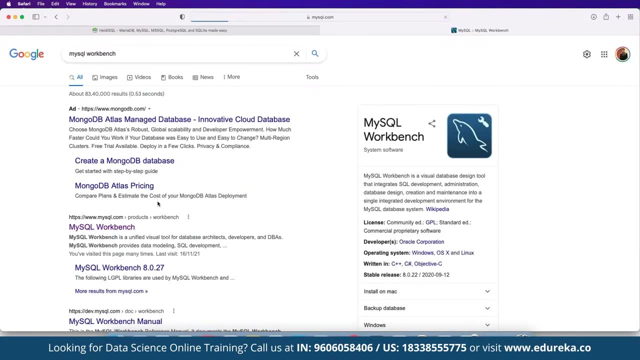 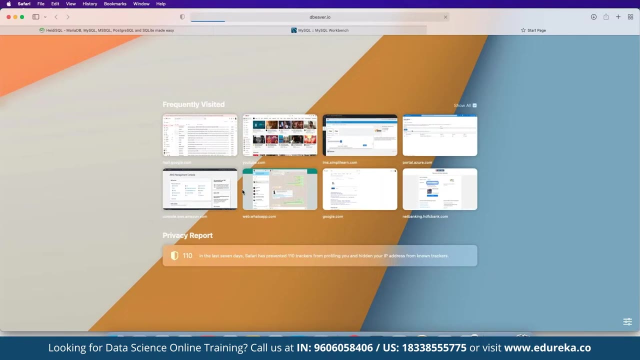 like we have mysql workbench. mysql workbench- if you want to get connected to a single platform through which we can get connected to multiple database sources, then you can also make use of tools, like we have dbver, so dbver is again one of the most. 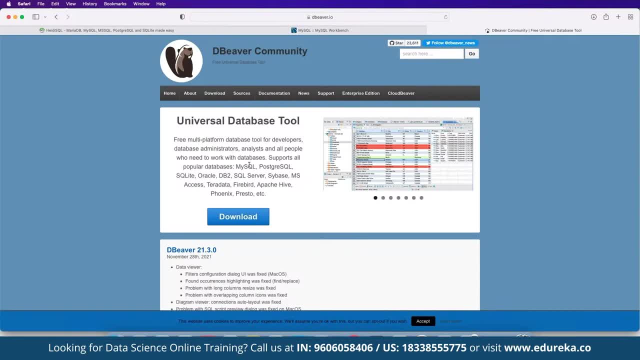 popular database engines out there which we can use to get connected to mysql, postgre, sqlite, oracle, telehealth, ms. access. that means to almost all the popular database engines out there. we can use it to get connected to them. so this is what we can define as a part of this setup. so 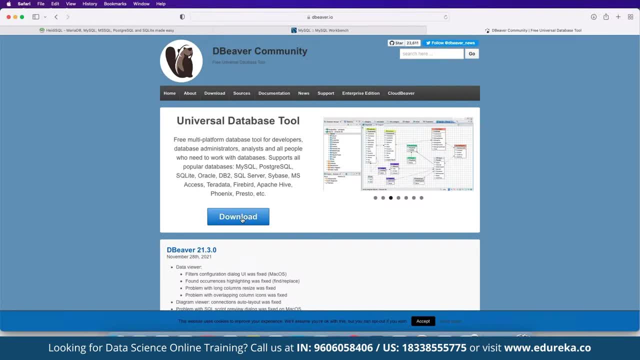 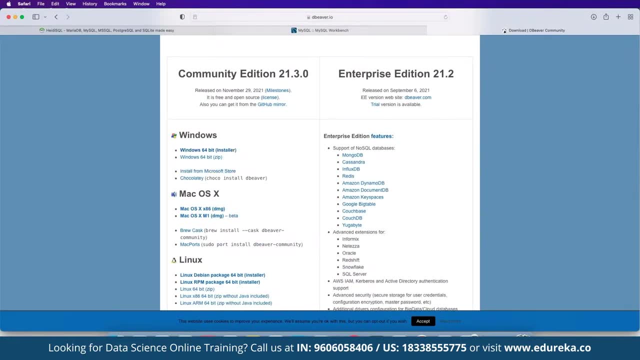 here we can go ahead and click on download, and here we can see that we have the dbver. we can choose to go ahead and go for the windows or mac os, based on the system that we have. let me share this url with you all so you can use it as a reference. 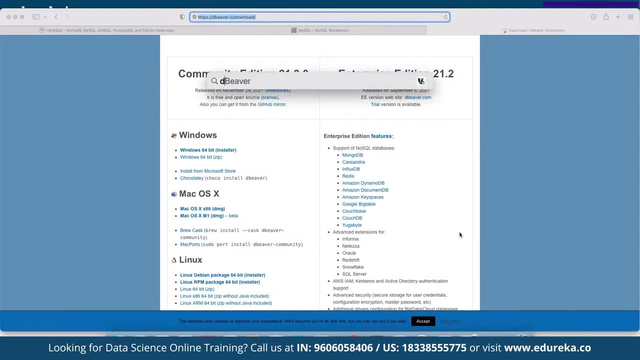 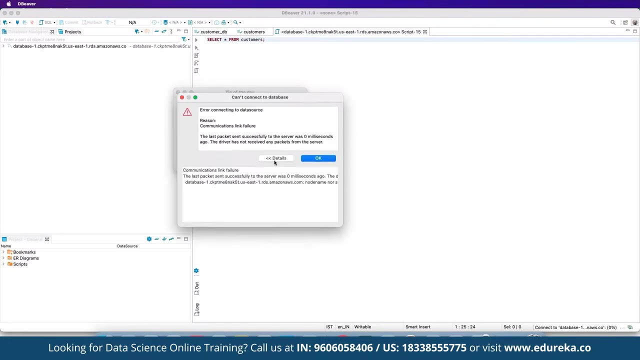 i'll share this in the chat window so we can all use it as a reference here and to get connected so we can open up this db work client if we have. so the best part of dbvo is it is offered as a part of the to get connected to the database that we have. so there is no licensing involved here. now this is. 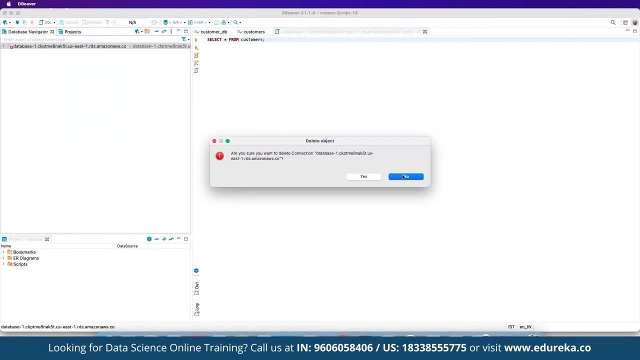 how the platform for db looks like, where we can start creating a new database from scratch and then we can start getting connected to any remote database and then we can view the data. we can perform all the credit operations we want. so what we can do is we can go ahead and click on this. 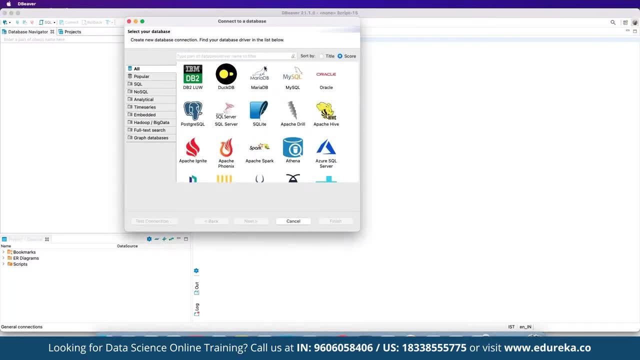 option which says new database connection, and here we can click on, here we can choose the database engine that we want to get connected to. for example, here we want to set up a connection to mysql engine. so we have the database that we have the access to is running on top of. 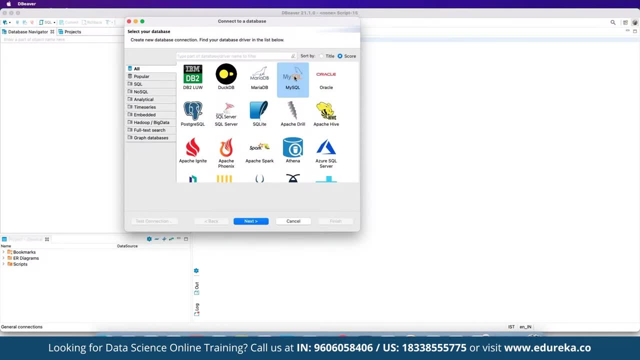 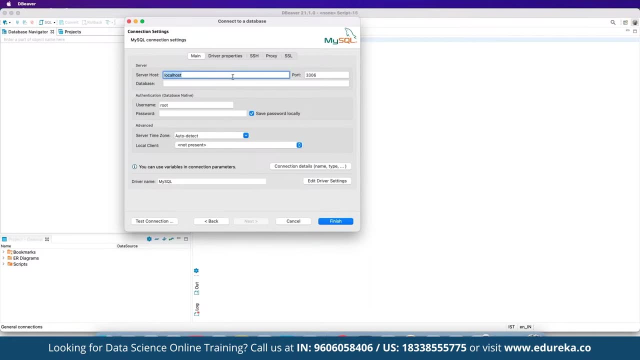 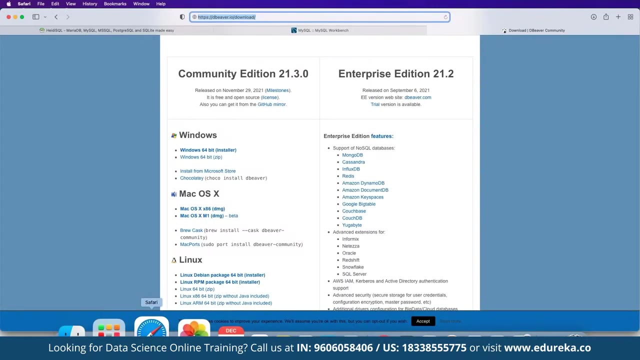 mysql database engine only and here we can click on next. now in here we can define the server host. so right now we want to get connected to a remote database engine. so we do have the endpoint that we can go ahead and get the access to. so this is the endpoint of our database engine that we want to get connected to. 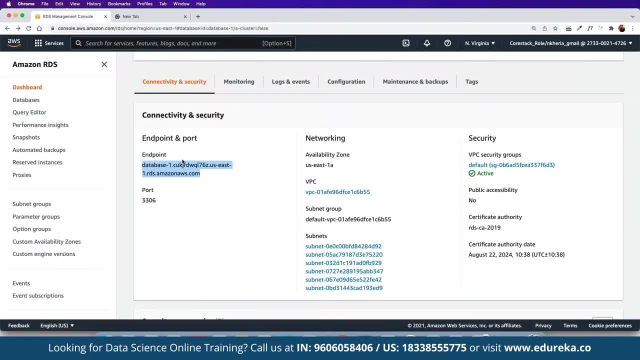 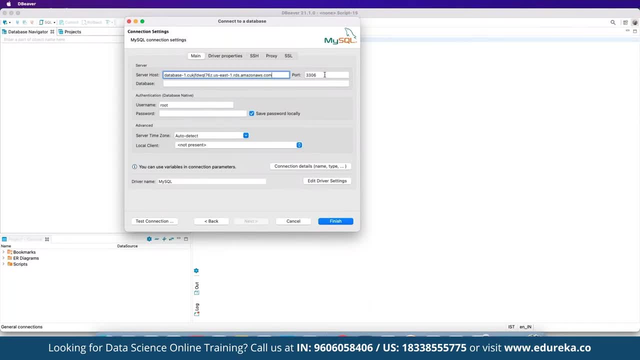 we have defined this on port 80 itself. so we have defined this on port 80, on port 3306. so this is a default port for mysql, just like we have default port for oracle, like we have 1521. so in case this port is already occupied, then we can. then we can define a different port whenever we are going to. 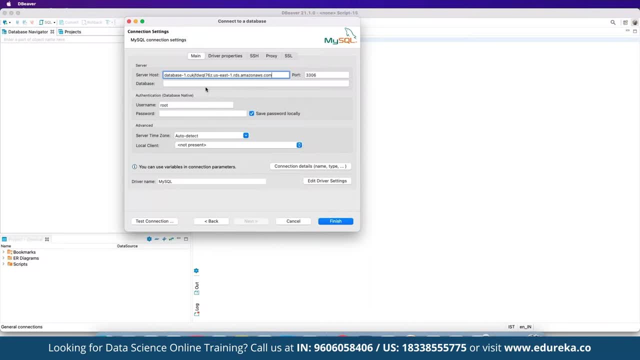 have the database engine and then we can define database name. in case this is a production level database and now we want to get connected to it, then we can find the exact database available. in this instance we can have multiple databases available in a given system. we can easily 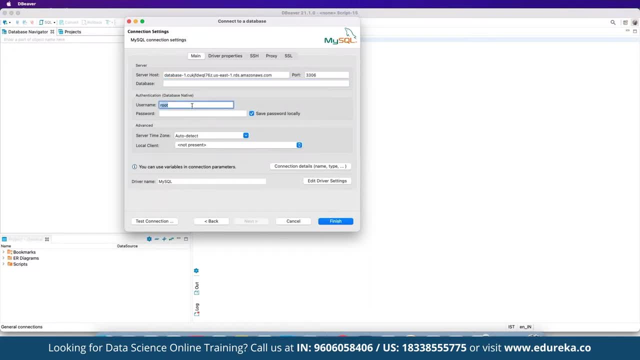 do that, then we have username, so username is going to be set. so at the time of deploying this database instance we had to find the username as admin and here we can set the password. we can test the connection, if we can, if the credentials are correct, if the port has been. 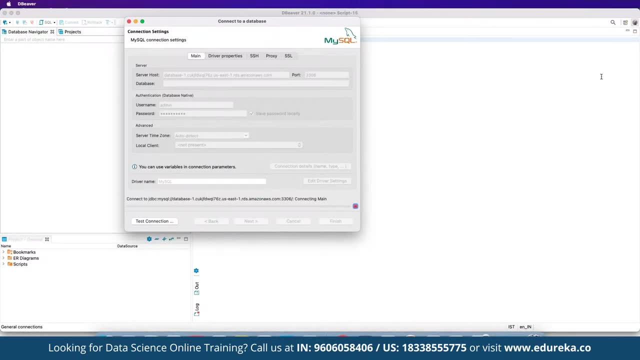 opened up, then we would be able to get connected. if not, then we have to check the firewall. for the database instance that we are trying to get connected to. the firewall should allow the access to the given port. it may take a while, all right, so for this given database, the public. 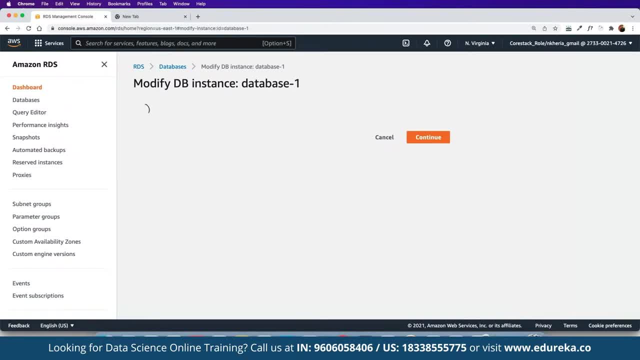 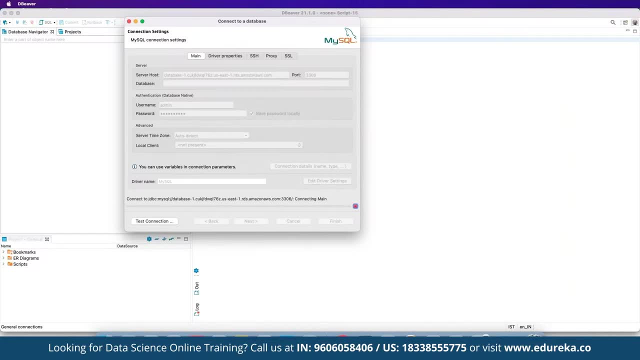 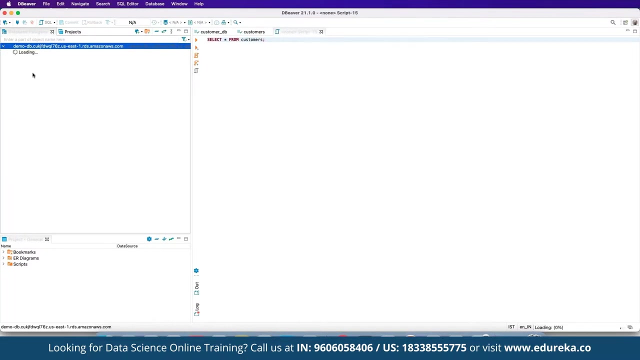 accessibility has been set to off, so we have to turn it back on just a minute because we have modified it. so it may take a couple of minutes for the connection to be refreshed once it is done and we would be able to get connected. all right, so the connection has been established, so now we can open up this database. instances. 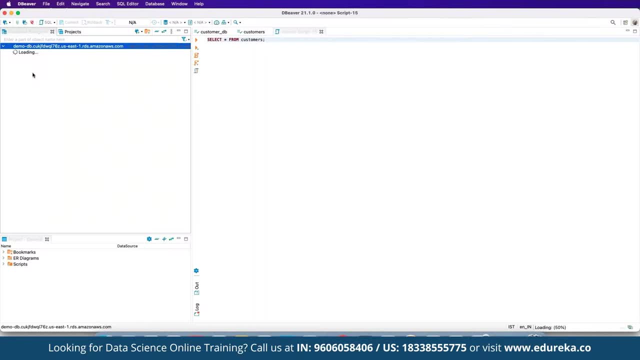 so this is the default database instance that we have, having default structure defined. so right now, since this is a blank database, so we don't have any anti-database instances up and running. so whenever we are going to run to work on this database based gui platform, either we can start manipulating the entire database by using the 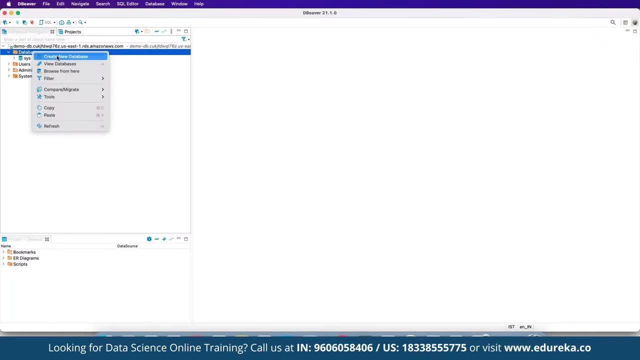 gui section, section here, like we have the create new database. so once we click on create new, so what exactly is happening in the backend? the sql script is being run, but again by using the gi platform we are able to create a database for us. for example, let's say, here we want to create a 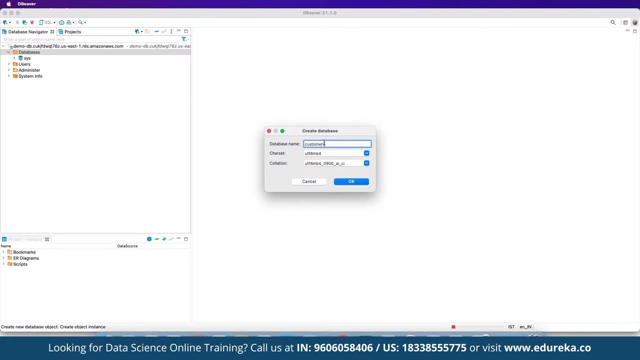 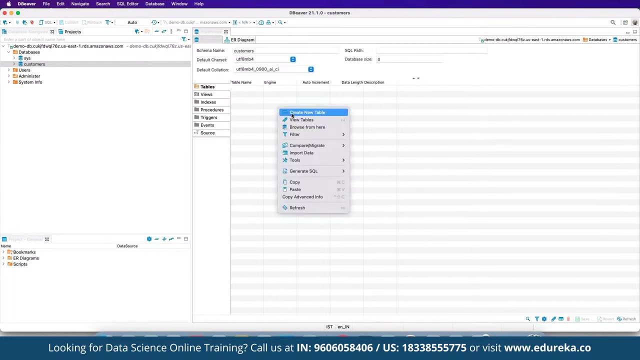 database by the name of supposedly customers. then we can see our database by the name of customers is going to be created. so we can and we can double click on this database and we can see the complete ui has been opened up. if we want to create tables, we can right click here, click on create new tables. 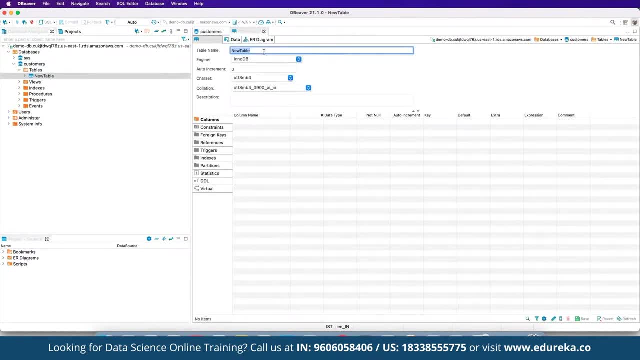 suppose here we want to find table for, let's say, here we have, for, let's suppose, for the info, and then within this we can create a new column. right click here, click on create new column. suppose here we wanted to find a column name. suppose as, let's say, here we have. 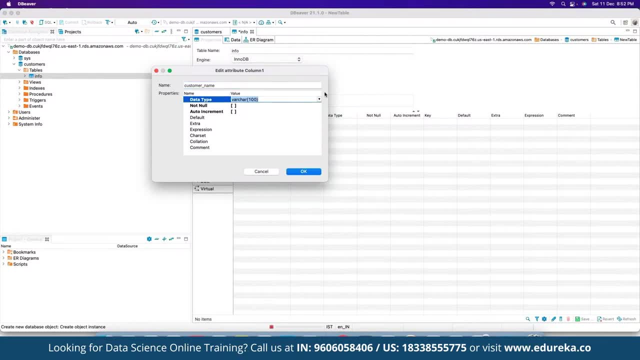 customer underscore name. then we can define the data type: whether we want this one to be based on varka, as in the string value or date time double float. so for name it is going to be for varka and then we can click on ok. again we can define new column. suppose this is going to 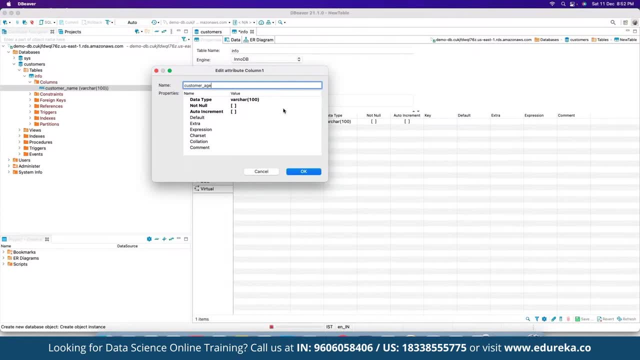 be for customer age. so here we have a customer age. we want this one to be not appear part of varka, but we want this to be part of the, let's say, the date boolean, or suppose a simple integer we can click on ok, and now, once we click on save all. so again at the end. 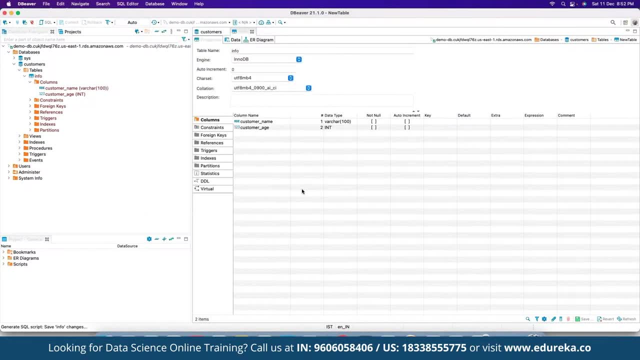 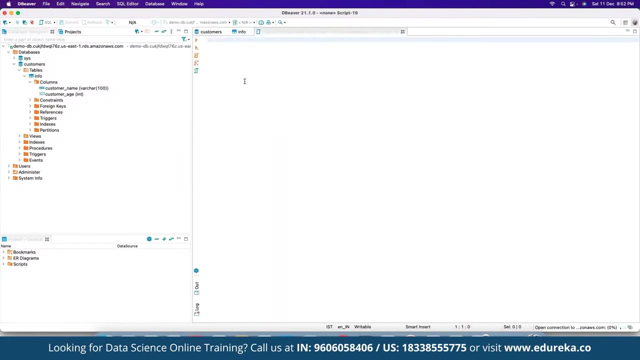 the sql script itself is going to be created here, then only it is going to be updated. so the main beauty of these different platforms is we. we can either use this entire gui or we can simply use the sql editor, where we can start typing the scripts directly. so what we do here is: 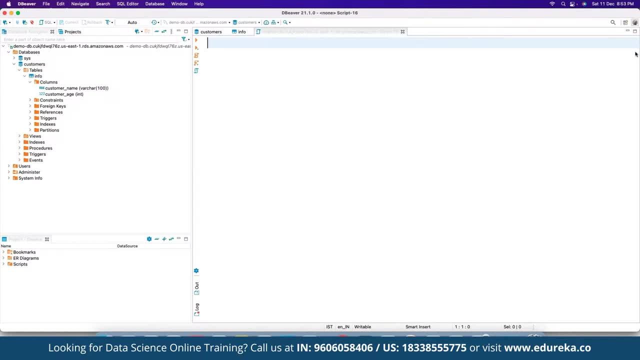 simply trying to generate the script back here. for example, let's say our goal is to create a database, our goal is to create a database, so we can simply run the script here. for example, here we define create database and here we can define name. suppose here we want to create a database. 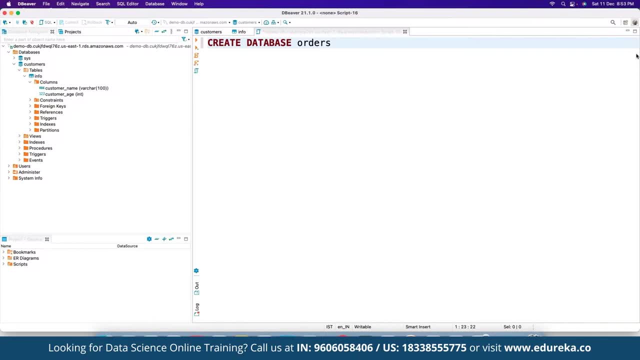 by the name of orders, then we can define the name as orders and then if you want to start using this database, then we can simply use the command as use orders in case you want to make use of this database we are going to create here. so this is simply going to create the database here, whatever name. 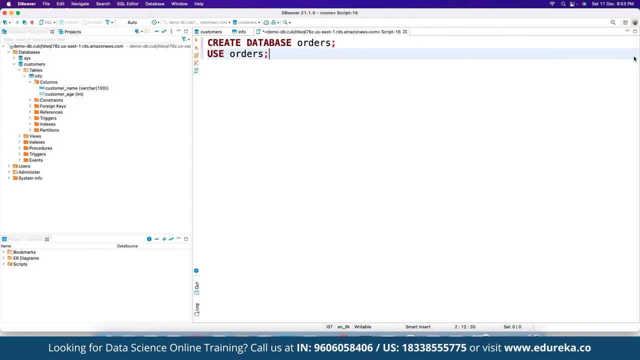 we have defined here and then we once we define the database. so, as you can see here, our database with the name of orders have been successfully created. the security has been executed. next, if you want to create a table within the given database here. so, first of all, if you want to, 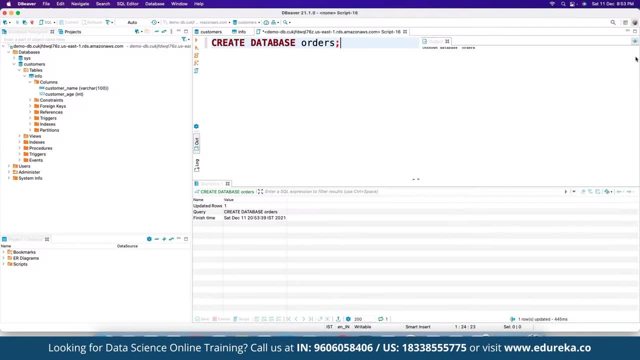 use a given database, then we can define use. suppose here we want to run all the queries on orders so we can use the table that we have defined. we can use orders so we can switch to orders and then we can start creating tables within the given query here. 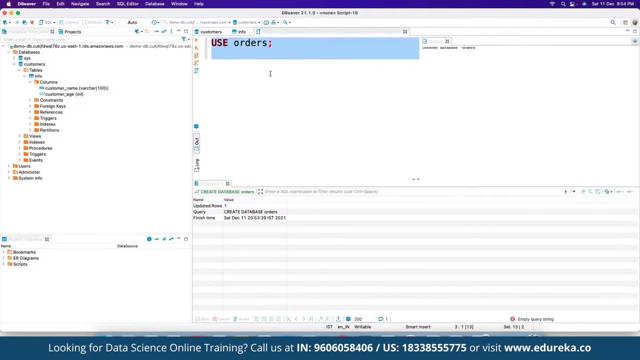 so, for example, now if you want to create a database here, so what you can do is we can go ahead and run the program as suppose: create table. let's suppose here we want to create a table for new orders, so here we can define new orders as what the name of the table that we want to create. 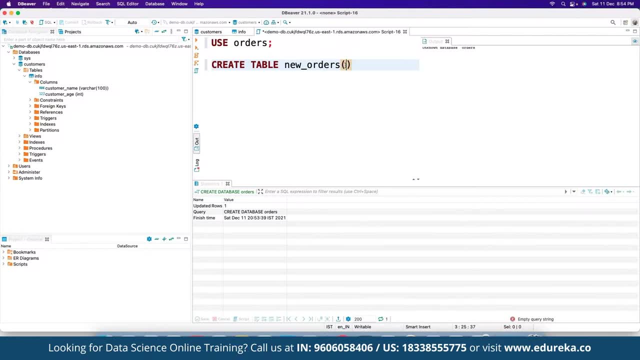 and then we can define the name and the data type of the variables, as in the columns. first of all we need to call the column suppose as customer. suppose here we can define customer underscore name, and suppose we want this one to be a varchar, suppose varchar of having. suppose this is 50 characters. we can define that. 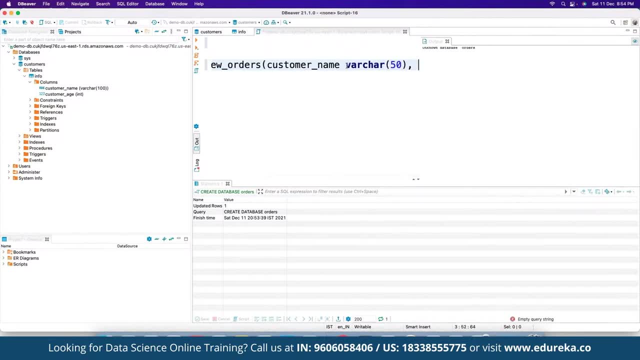 varchar, and then, and then we can add a comma. then suppose next we want to have, let's say, item being added, so again we want this one to be varcat, having suppose as 50 characters. then again we can define: suppose we have price, and we want price to be part of, suppose, a double, and so we 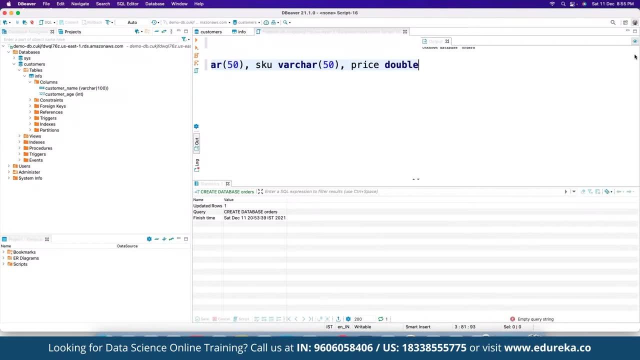 get what we're doing here. we are simply defining the values, so we want to have a double or float or whatever values you want to have. now, once we are done, we can simply go ahead and execute the script here. so now a table by the name of orders table is going to be created within the same 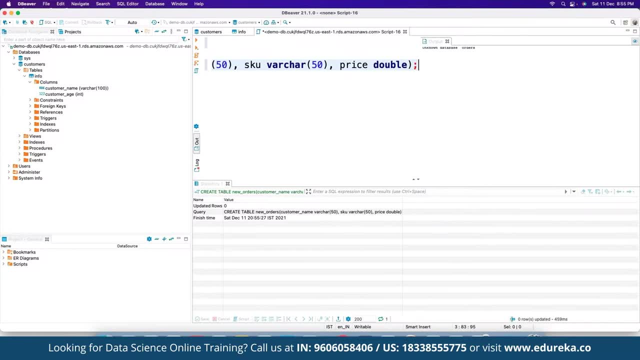 orders table that we have defined here. so what we are doing here, we are simply creating a script. we are simply running a script and based on these scripts, only the data is going to be updated. so now, if we refresh our left sidebar, we can see we have orders on our tables, we have a table. 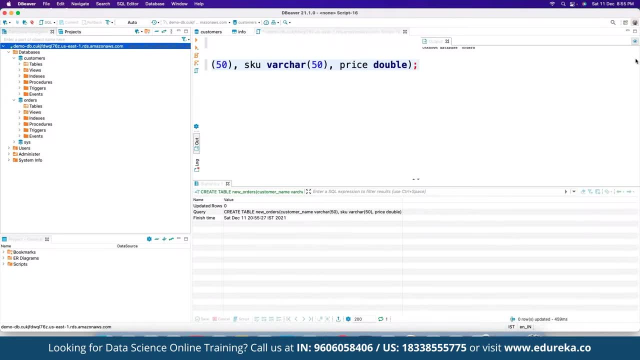 that is going to be created with the same entries that we defined here. so whatever we do, that is going to be updated and that's how the entries are going to be there, based on whatever values we have defined here. so now, if we refresh our left sidebar, we can see we have orders on. 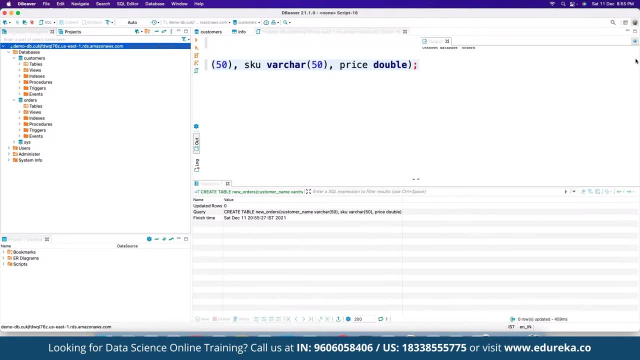 here. so, whatever we are going to create, that's how it simply works. and now, if you want, if, in case, we have certain entries- of example, suppose, we have certain entries that we need to be, that we need to work upon, so here we can go in and define the entries, and they are going to be defined. 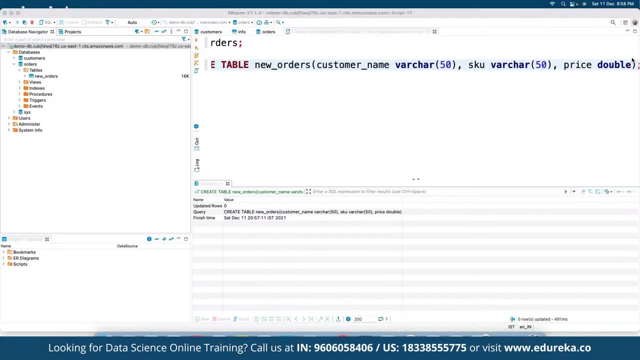 accordingly. that's how it works. and then we want to insert values. so here we can use the insert into the name of the table that we wanted to define, and then we can define values. as for the table structure that we defined here, for example, now we want to run a simple insert into. so here we have insert into. now we want to insert into. 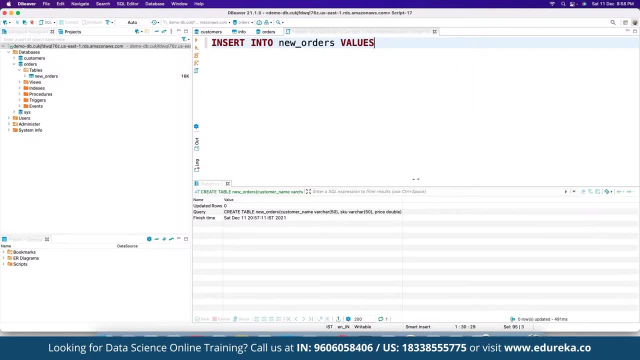 new orders and then we can define whatever value we want to enter. so we have so, under new orders, what we have here. we have customer name sq and the price. suppose the customer name is going to be jane, then the sq is going to be supposed to say s101 and then the pricing is supposed going to be.